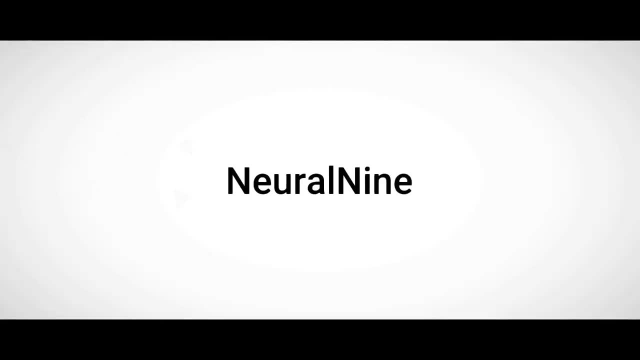 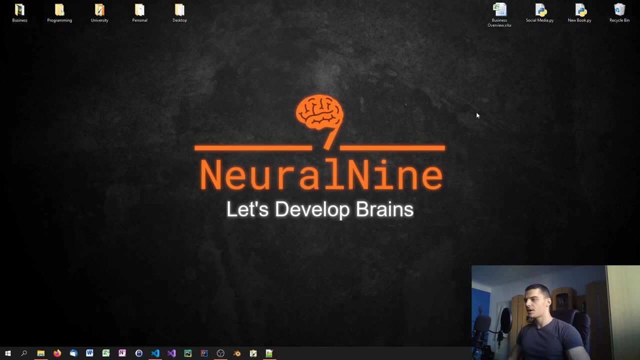 What is going on, guys? Welcome to the fourth episode of the C++ tutorial series. In today's video, we're going to talk about variables and data types, So let us get right into it. All right, so, as always, let's start with the code structure First. we're going to say include: 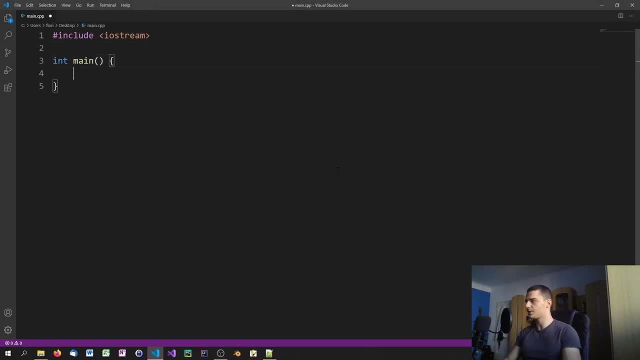 IO stream and then we're going to define our main function here: return zero. And before we get into variables and data types, one thing that I want to show you is that you can also use the whole std namespace that we used in the last video. So what we did is we said std cout and then 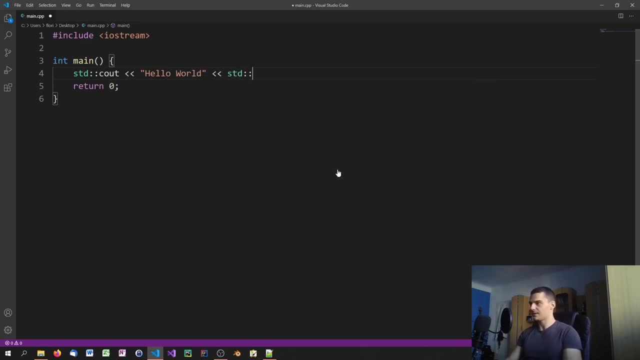 hello world and std endline. This is what we did, What we can also do if you don't want to always specify that std namespace in front of every function or tag or whatever you're using out of those std prefixes here. However, why didn't I show it to you in the first video is because I 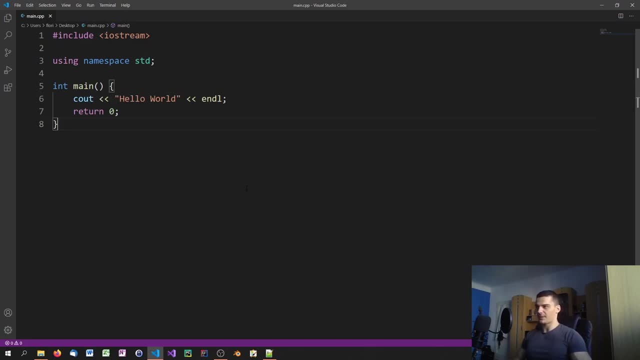 don't think that you should get used to that way of programming, because using namespace, std and then just writing cout and endline and so on is not considered to be best practice. I mean, of course, you don't always have to code in best practice and it works. You can definitely go ahead and 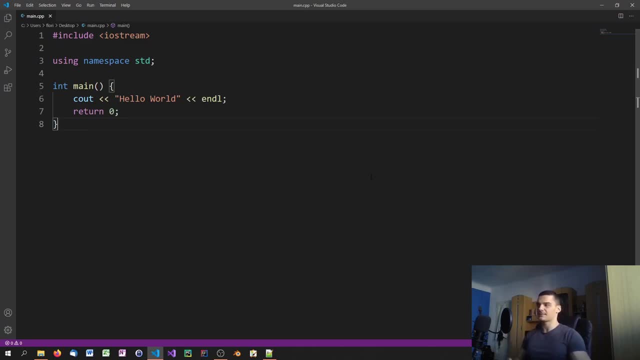 write code like that. But if you're going to write clean C++ code, you're not going to do it like using cout and endline from std right now And it doesn't make sense to use the whole namespace because of that. If you're only using cout, endline, maybe one or two other things, it doesn't. 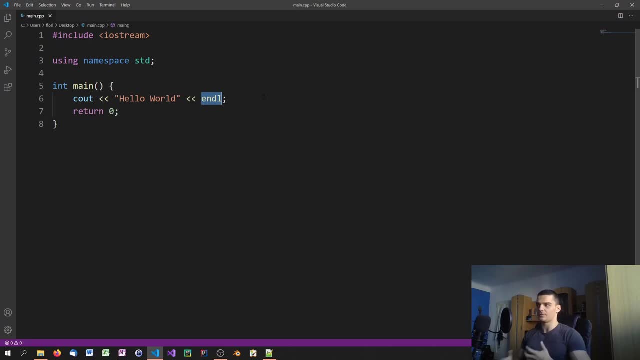 make a lot of sense to use a whole namespace to just include or import or whatever, to just specify that you're using the whole namespace, because it's just too much so to say It's not clean, It works, It doesn't have any problems, It doesn't bring any problems into your program. yet 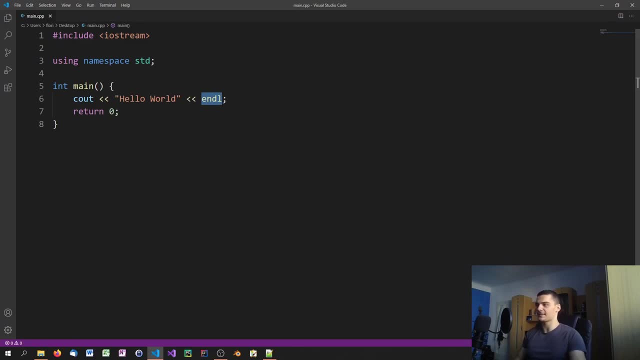 unless you know you have a second namespace that also has something like cout or endline, Because then you run into some problems. But it's just not the general accepted best practice way to say using namespace std and then cout and endline. You're always going to see this in code. 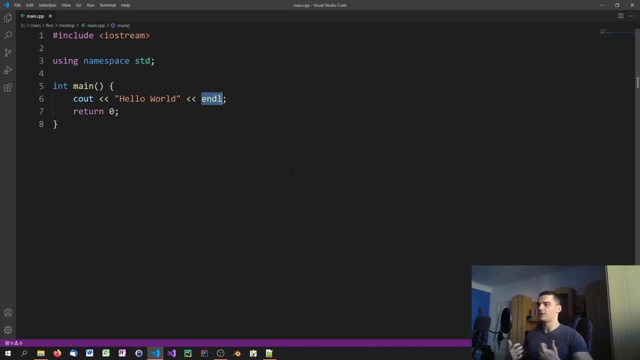 examples, because it's just more convenient. And if you're doing some videos, if you're writing a blog post, if you're just practicing, if you're just writing some sample code, you can definitely do it like that, And we can also definitely do it like that in the tutorial series here. I'm not 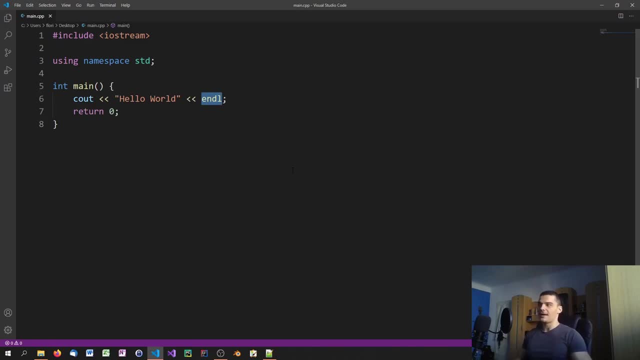 going to do it like that, But we can do it because it's not wrong. I don't want you to get used to that way of programming, So we're not going to do it like that. I want to show it to you that it's possible, But we're going to write the best practice. 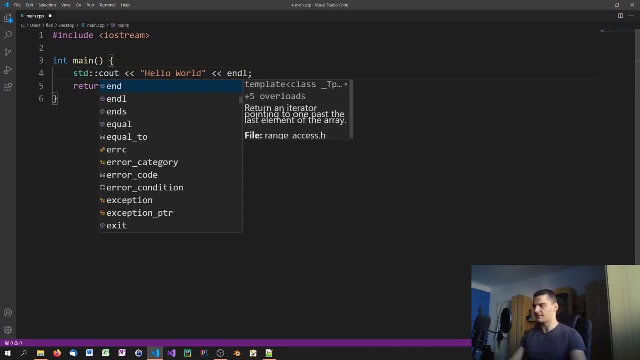 type of code here. We're going to always specify std before we use something from that namespace. So that's just something I want to show you before we get into variables. All right, so let's talk about variables Now. variables are essentially just placeholders for. 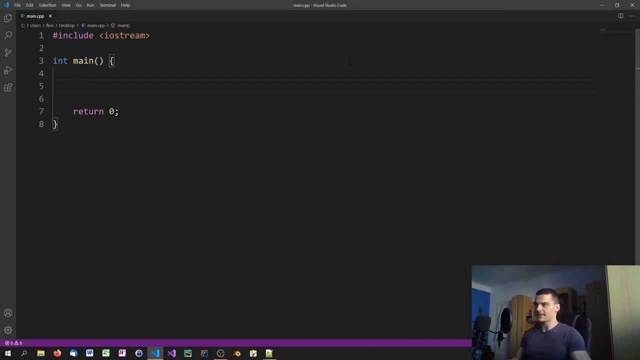 values and programs. So you know maybe variables from mathematics. already they're just stuff like x equals 10, or y is a function, or y is some list or some set or anything in mathematics. And it's the same way in programming, just that we have a lot more data types, we have integers. 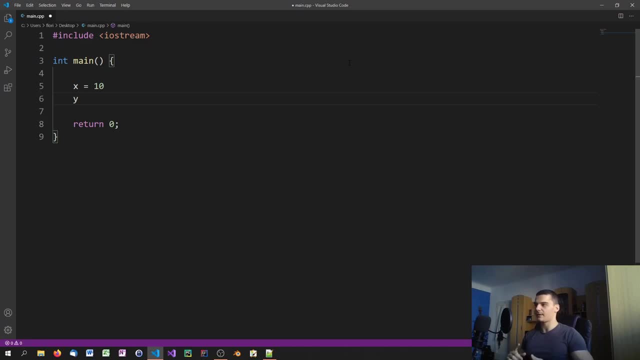 so whole numbers, we have floating point numbers, we have Boolean values, you have text values, you have lists and collections and structures And, later on, even objects, whole objects that represent stuff, like a person, for example, can be stored in a variable And, in contrast to, 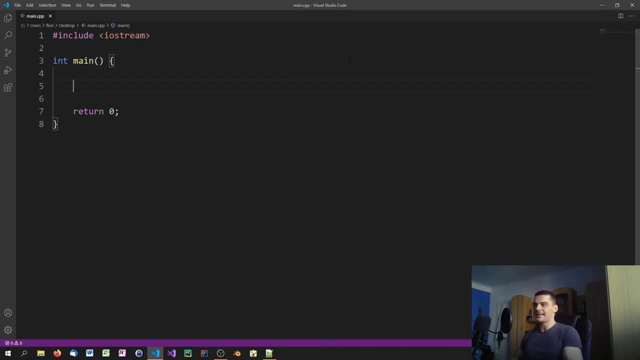 languages like Python, for example, C++ is statically typed, which means that we have to specify the data type of a variable before we can actually assign a value to it. In Python, for example- for those of you who know Python, you know that you just go ahead and say a equals 10.. And then the interpreter already. 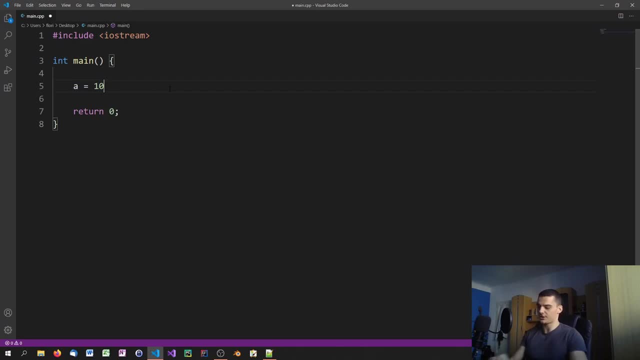 knows that a is going to be an integer for now And later on. you can also say: a equals something else like hello. So hello is a text. So a is no longer an integer. a is a so called string, And in Python this works. In C++ we don't do things like that. 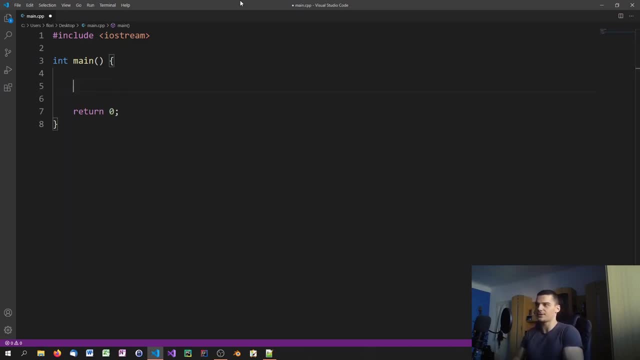 In C++, what we do is we specify the data type first, And if you want to have an integer, you specify the keyword for the integer, which is int, And then you specify the variable name. So you say int x, for example, int x equals, and then you can say int x equals 10.. And if you want to, 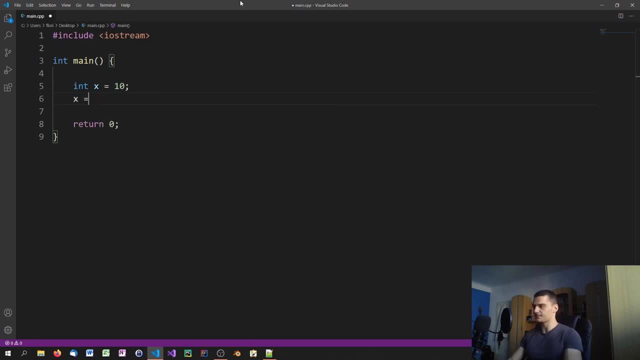 change the value of x. what you do is you just say x equals 90. Again, don't forget the semicolon for those who are used to Python, And you can change the value as many times as you want. Of course, you can say x equals 20.. 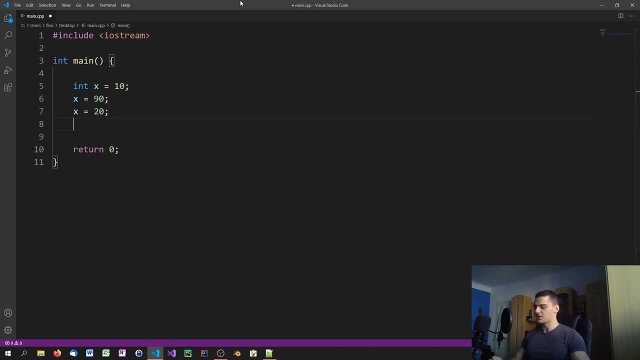 x equals 90. But you cannot change the data type. you cannot just go ahead and say x equals hello, because then the compiler will tell you that this type is not compatible. you have an integer and you want to assign something else to it. This is not an integer here. you want to. 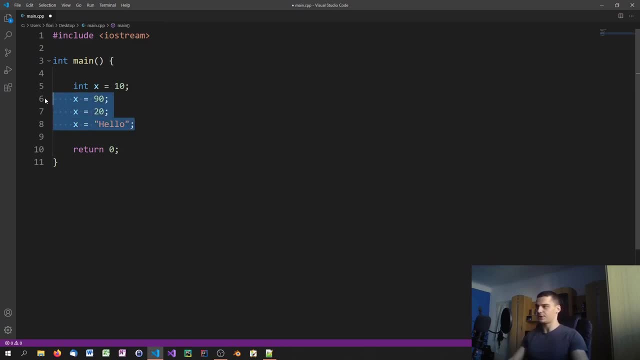 assign a string or something else, but it's not an integer. it's not compatible. So this is statically typed. you have to specify the data type first, and then you can assign a value to it. So that's not too complicated. But let us now go ahead and talk about the different. 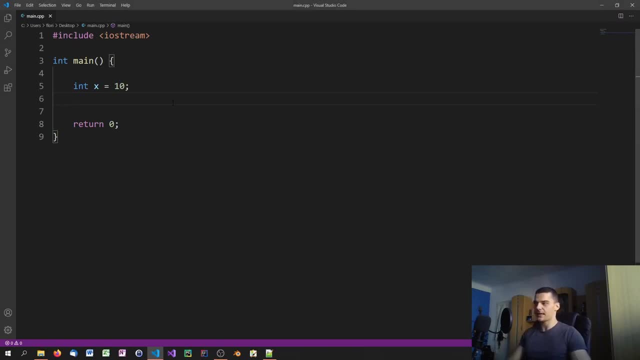 data types And we're going to talk only about the primitive data types. Now, this means just basic stuff like numbers and texts and Boolean values, and not stuff like lists or structures or classes and objects. So just the primitive data types here And we're going to to subdivide. 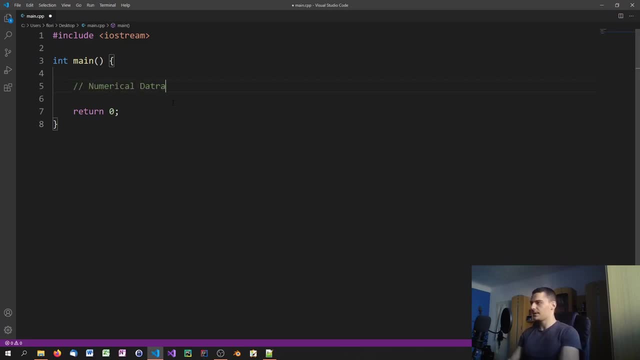 them into three categories: First of all, the numerical data types. Second of all, the textual data types. by the way, these are just my terms, So maybe they're not 100% scientifically accurate. And then we have the Boolean. Okay, so the numerical data types are essentially, you have. 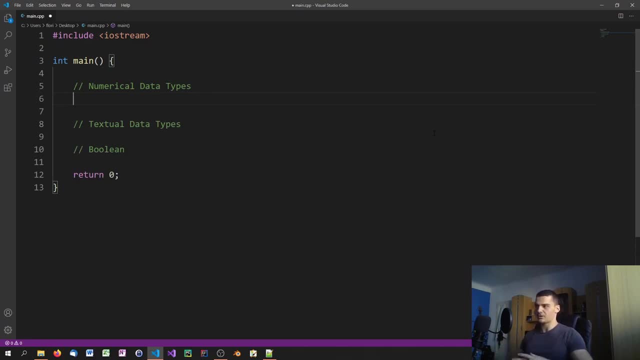 either whole numbers or floating point numbers, But there you also have different types of floating point and different types of whole numbers. So you have the integer- this is the basic one that we saw already. int i equals 10,, for example. But then you also have the short and the long and the 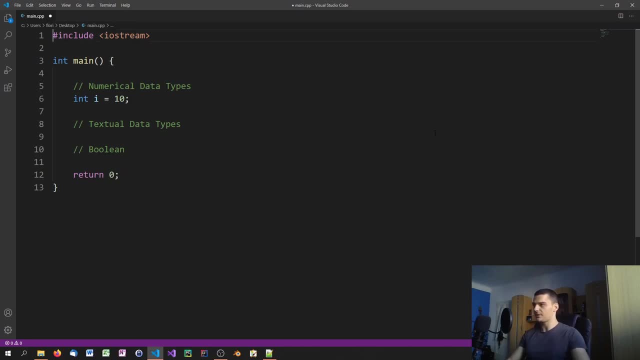 short and the long are actually just integers. In fact you can, you don't even have to say just short. you can say short s equals something, But you can also say short int s equals something, And that's actually the same thing, because short is just another type of integer And the only difference is the memory. 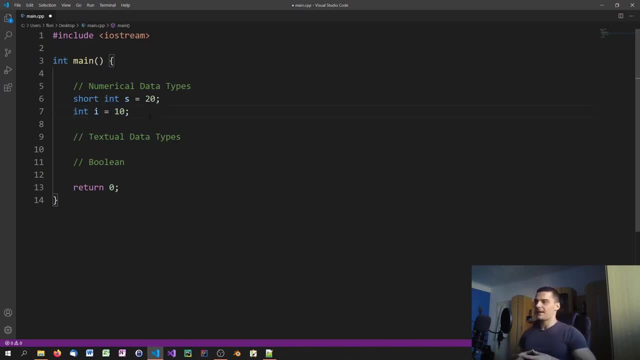 value or the memory amount that they occupy. Now, this is something that you never worried about in Python, because in Python you just you know, you define stuff and it happens. In C++ we're operating on a lower level And this means that we need to care about stuff like memory management. 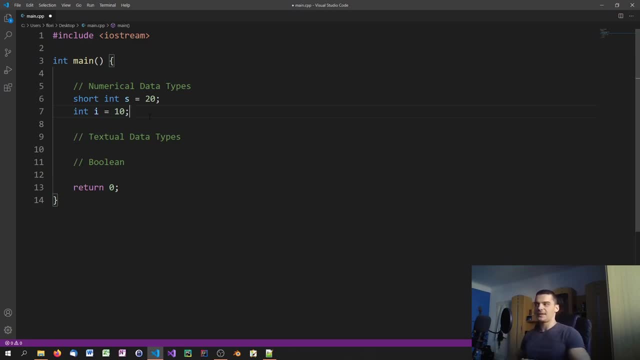 we need to know: do I really need an integer, Or is a short enough, maybe? The difference, of course, is that they occupy a different amount of bytes, So we can actually look at how many bytes they occupy by using the size of function. 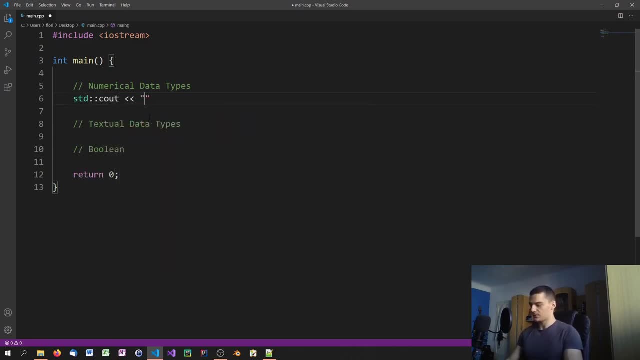 So we're going to say std cout And then we're going to say integer int. So this is just some text. you can write whatever you want in here And then you say size of int And then maybe an end line in the end. So what this function is going to give you here is 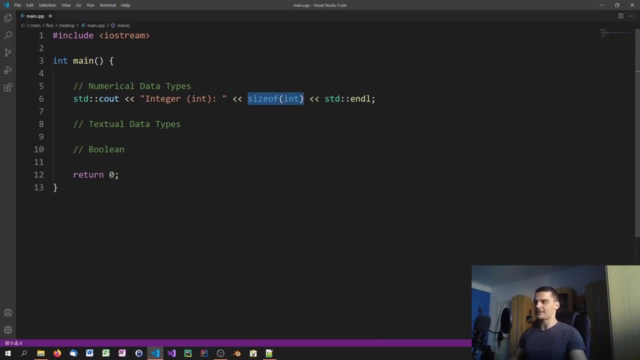 it's going to give you how many bytes an integer occupies in the RAM, in the memory, And we can go ahead and open up a new terminal and compile this maincpp mainexe And then we can go ahead and run mainexe And you can see that we get four. 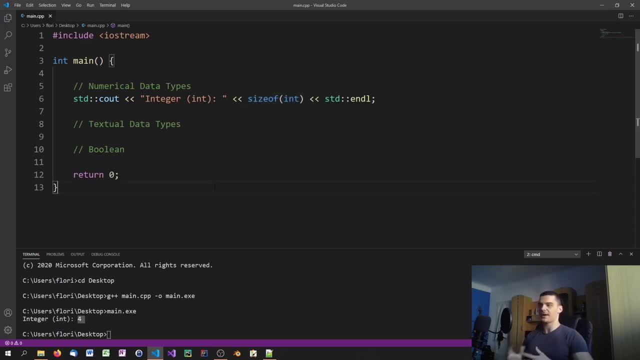 this is four bytes and a byte is eight bit. I'm not going to explain the binary system to you. If you know the binary system, you have essentially one byte being eight bit, which means that four bytes are four times eight bits, which is 32 bits. It's quite a large number. 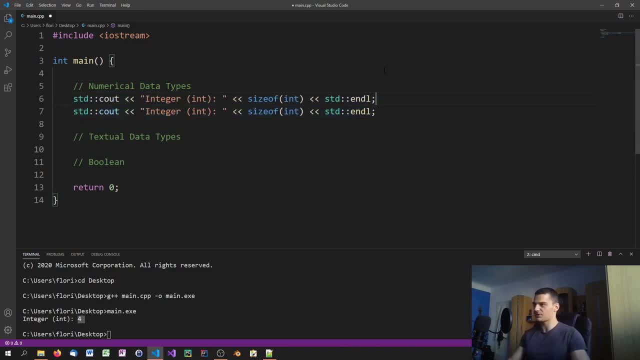 And we can go ahead and do the same thing here for the short And you're going to see that a short occupies less amount of memory. So we can say short, short, size of short can also say short, int doesn't matter. And then we compile it again and run it again And you can see a short only. 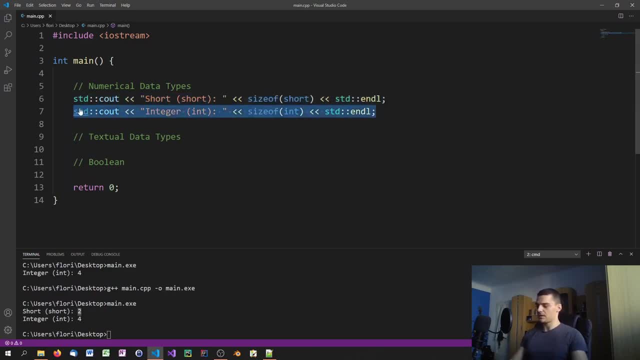 occupies eight bytes. We can do the same thing for long as well, And there you will notice something that's quite interesting, And it is that in C and C++ oftentimes things are just not defined. Now, in this case, in my computer, it's going to say that: 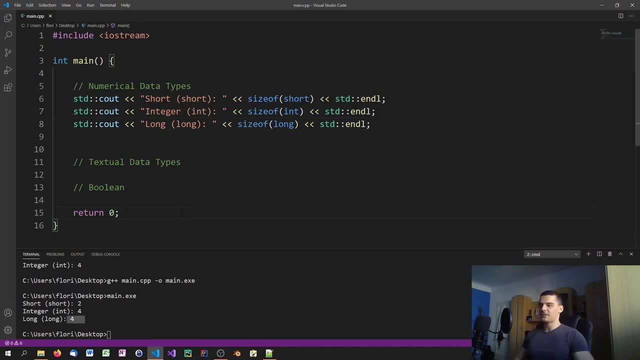 along also has four bytes. doesn't have to be that way. on your system The definition for along is only that it has at least as many bytes as an integer. doesn't mean that it has to have more. it can have more, but it has to have at least as many. So maybe in your computer it's going to be: 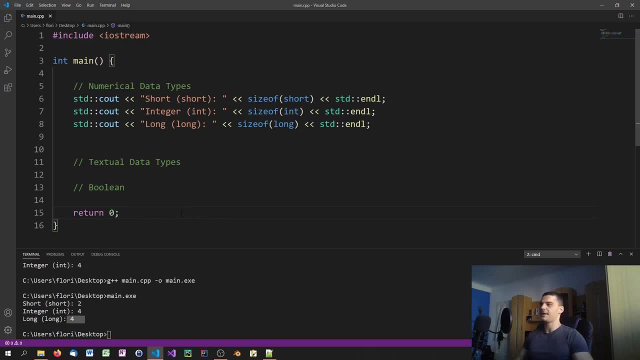 going to have eight, maybe it's just going to have four, it doesn't matter. It's not defined and we'll encounter and encounter many things in C and C++ that are not defined, that are undefined. we don't know what's going to happen when we do them. they're not forbidden, we just 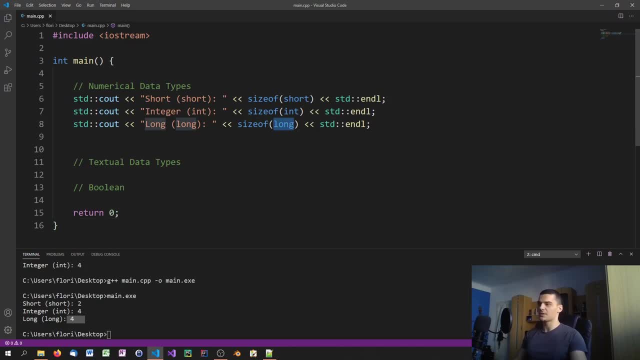 don't know what's going to happen, And this is also one of those. we don't know what size of long will return on every system. So what does that even mean? What does it mean that a short has two bytes and an integer has four bytes? For this we're going to open up the Windows calculator. 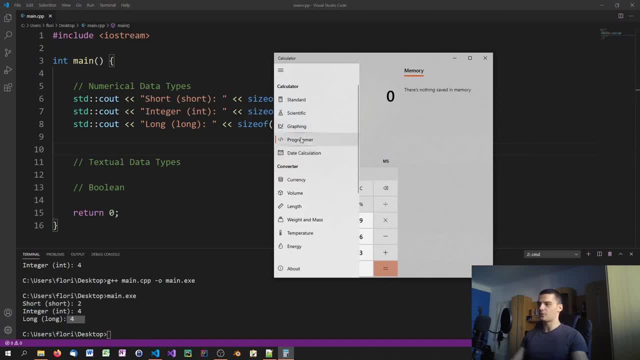 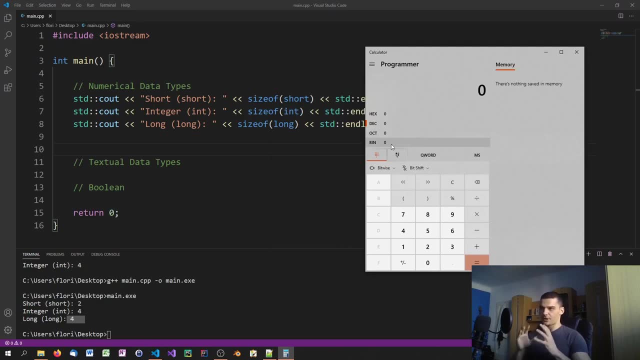 so just open up your calculator and set it to programmer mode And then we can talk a little bit about the binary system. we're not going to explain the whole binary system, So if you're not familiar with it you can just ignore this part or just watch it and accept it as a truth. But 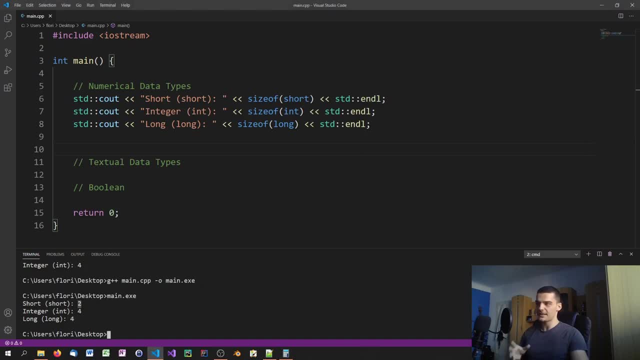 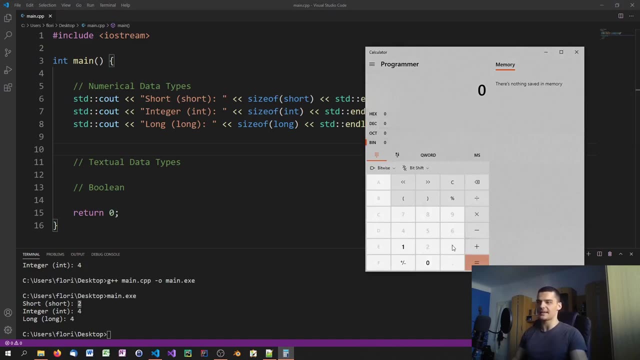 essentially, if you have two times eight bits, or two bytes, two times eight bits, you have 16 bits, And 16 bits means that you have 16 zeros and ones that you can set, which means that you have a certain range of values that you can set. So, if you have a certain range of values that you can 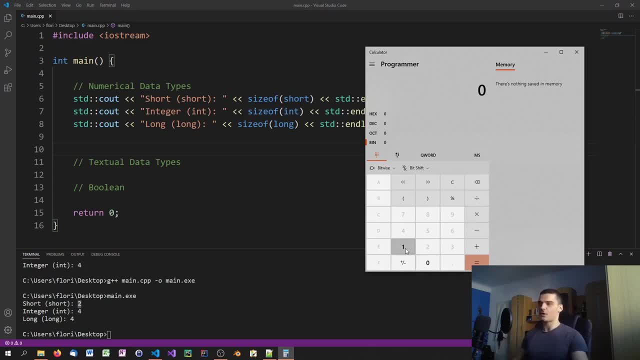 use for this short. So, for example, if I set all the values, so all the individual bits, all the 16 bits, to true, I would have 1111,. this is four, then we have eight, then we have 12. And then we. 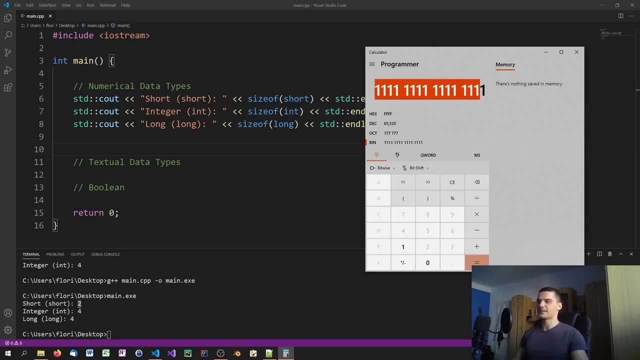 have 16.. So this would be 16 bits set to one, And if you convert this number to decimal, you can see that that is the number, That is the maximum number that we can represent using 16 bits, using two bytes. Now we can go ahead and set the value of 16 to one, And then we can go ahead and set the. 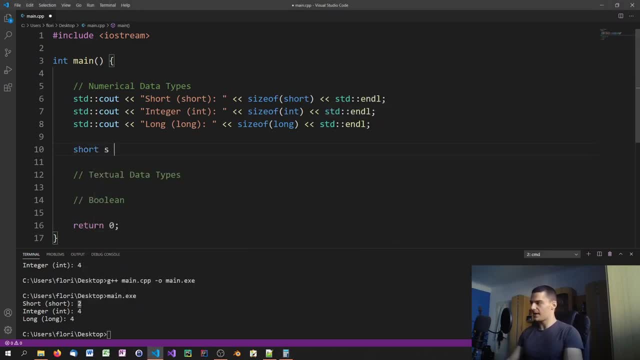 value of 16 to one, And then we can go ahead and copy that number And we can say short as equals that number without that here, And we can go ahead and print it, But you're going to notice an odd thing here. So I'm going to say actually just as itself And line you're going to notice. 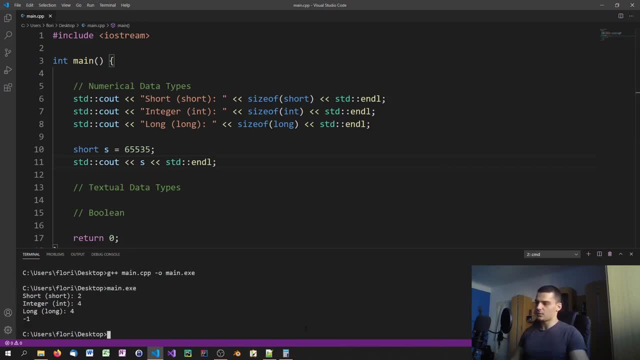 something that's a little bit odd here. it's going to not work the way we want it to work, because it's going to give us minus one, And even if we decrease it or increase it, it's not going to give us what we want. And then it's going to give us minus one, And then it's going to give us. 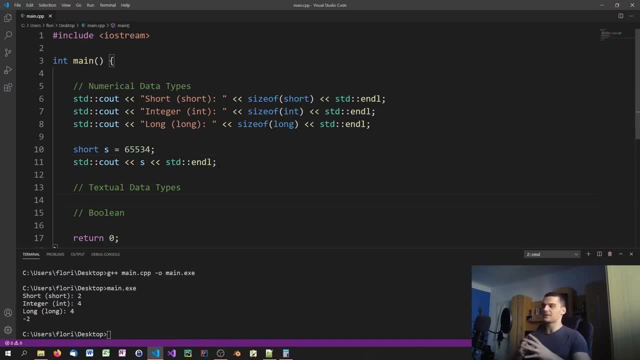 minus one, And this is because we're not using a so called unsigned short. The difference between a signed and an unsigned short is that if you have a signed number like that, this is the default. we don't need to specify it. But if it's signed, this means that we start at zero and we go into. 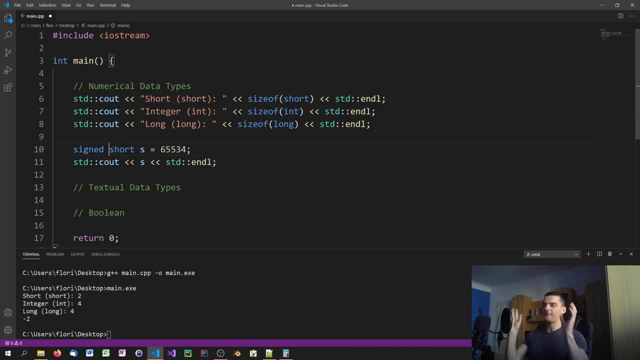 the positive direction into the negative direction, have as many bits as we can. so to say So, instead of using the numbers- zero to that maximum number here- what we do is we go from zero to half that number and to from zero to negative half that number. I hope this is not too confusing. If we want to use all 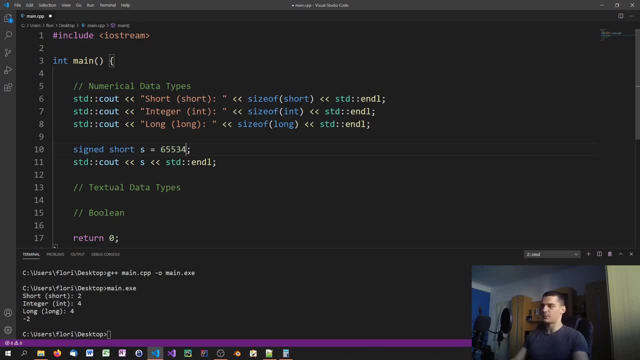 the 16 bits only for positive numbers in C++. what we do is we say unsigned short, because by doing that we can use a full range from zero to 65,535.. So we can go ahead and compile this and you can see that we get that value. And then we can go ahead and compile this and you can see that we. 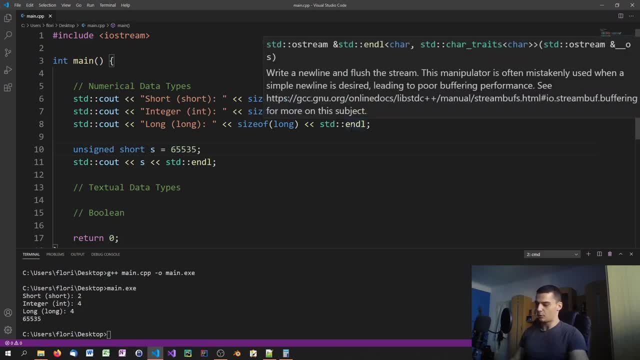 get that value, And then we can go ahead and compile this, and you can see that we get that value, And then we can go ahead and compile this and you can see that we get that value. And now, what happens if I add one more to it? What happens if I go beyond that number and try to add one additional? 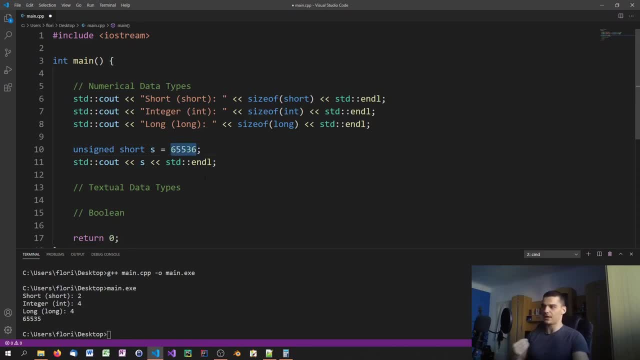 bit, Because, in order to represent that number, 16 bits are not enough. We need to add one more bit. What happens if I try this with a short that only has two bytes? You can see what happens: Actually, it stops. Actually, this is not what I expected, because 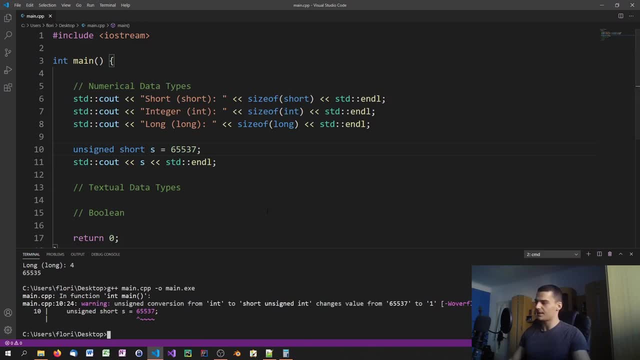 usually it gives you an overflow. Oh, it didn't compile, that was the problem. Yeah, as you can see, we're going to have a warning, a compiler warning that says: overflow something with overflow. This means that we're going beyond the limits. This means that we're going beyond the capacity. 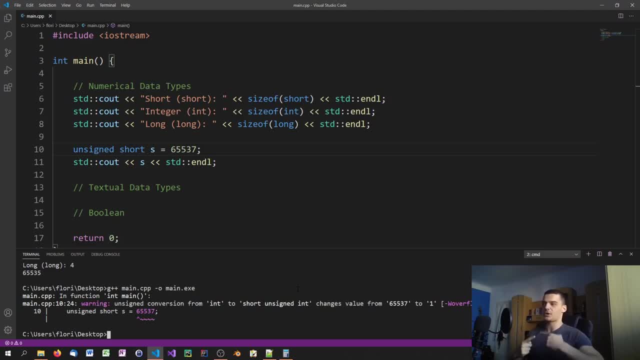 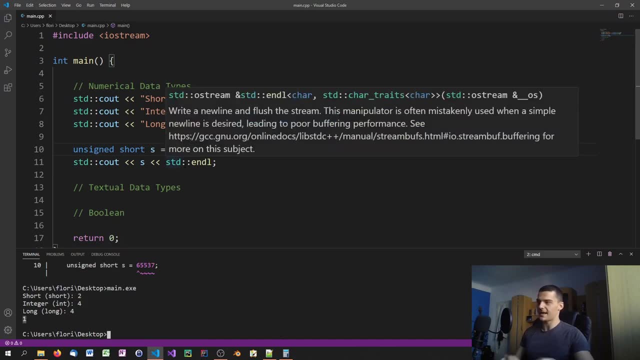 that we have And instead of saying no, you cannot do this, it's going to just overflow, So it's going to start counting from the beginning again. So if I run this, where is it? There you go, you can see, I get one because I surpassed the maximum by two. If I surpass it by one, 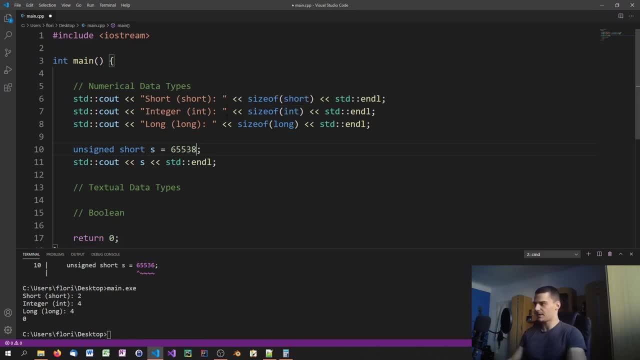 and if I surpass it by three, so if I say eight here, we're going to get two. So it just begins. it just starts all over again Because it doesn't have any capacities. it just has two bytes And if you try to store a number that's too high into it, it's going to overflow And, of course, 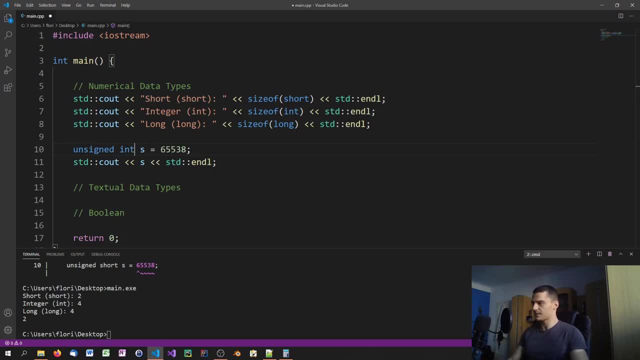 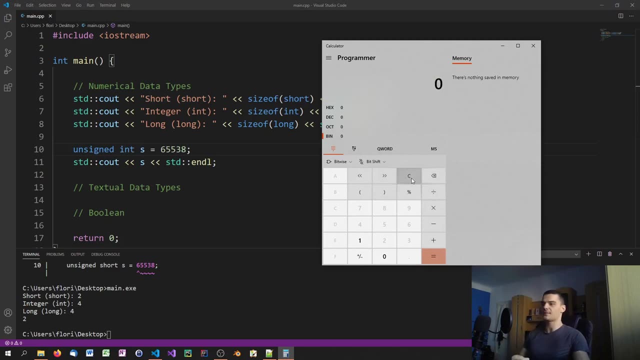 this can be done for integers as well. we can go ahead and say unsigned int And we can think about what this means. We have four, we have four bytes, which is four times eight bits, And instead of doing this in binary, we can just say F. F, as you can see, is four ones, So R is one. 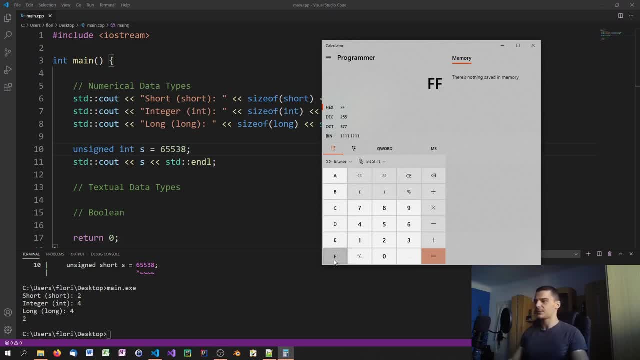 or f is half a byte when you're using it in hexadecimal. So we can say F, F, F, F. So we have two bytes Now. then we have three bytes and four bytes. So this is the maximum number that can be represented with an unsigned integer. Let's see if that's true. 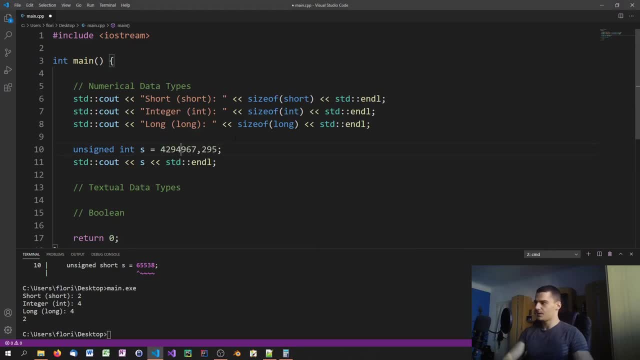 we can say: unsigned int equals that number And we can run the script, the program always making that mistake, and you can see that this number is represented correctly. and if i go ahead and say six here, so one more than is allowed, you can see i got a warning here and 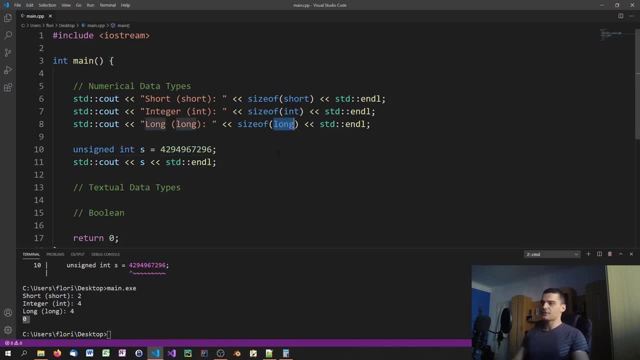 we start at zero all over again. uh, for the long. it's going to be the same on my computer, since it's also four byte. but what we can do, if we really need uh more, we can go ahead and say long, long. i'm not going to change the string left here, so just ignore it, but we can go ahead. 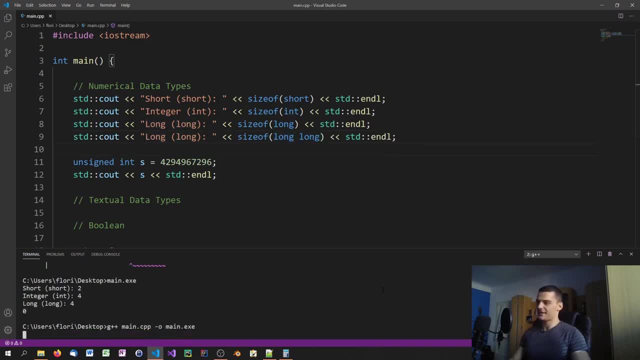 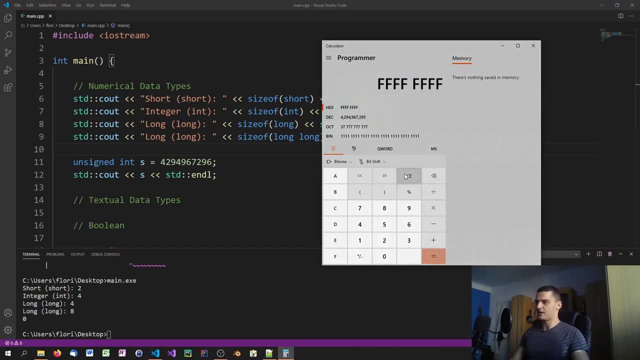 and try a long long. this is something that is going to have a little bit more um space. as you can see, it has eight bytes and we can go ahead and see what eight bytes are. eight bytes are essentially one, two, three, four, five, six, seven, eight and, as you can see, the windows calculator. 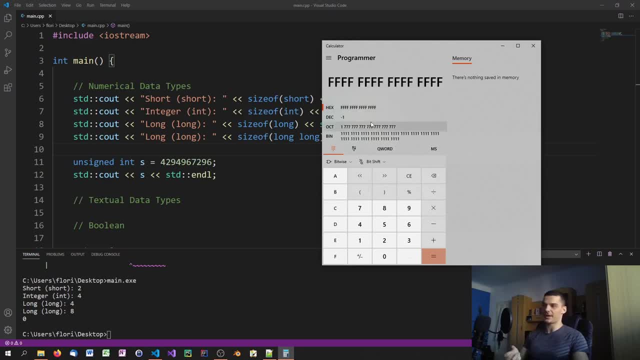 itself gets an overflow because that's too much. it doesn't store anything that's more than just a long bomb, um. so we're not going to to do the same value thing here, but essentially it will give us a different value for each of the two, but it's really important. 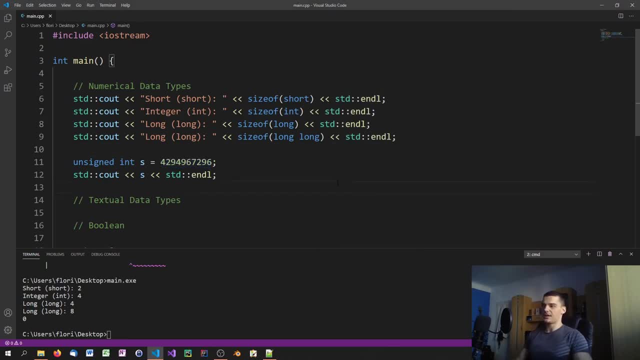 that it can have that same value. uh, Essentially, if you really need a lot, you just say long, long. Otherwise integer should be enough for most calculations. But you can see that in C++ we need to worry about that. In Python you can just define any number and it's going to adjust. 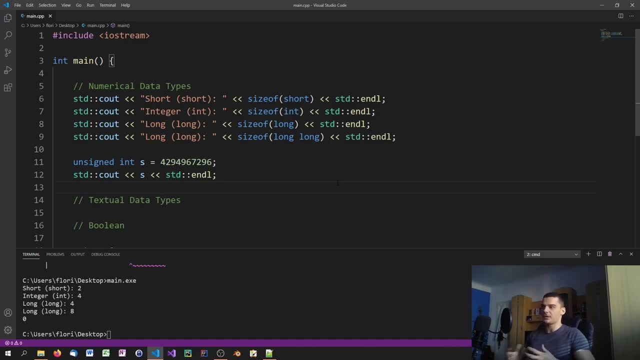 and it's going to allow you to have that number, no matter how high it is, how large it is, as long as you have enough memory left in your RAM, of course, But this is something we actually need to take care of in C++. 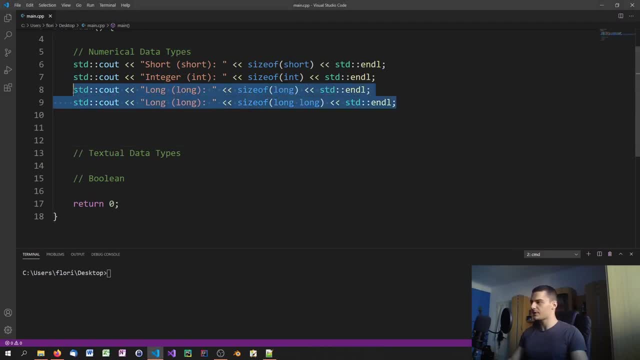 All right. so besides those whole numbers here we also have floating point numbers, And for those we have the two data types, float and double, whereas the float is less accurate and the double is more accurate. So the double has, I think, eight bytes double. 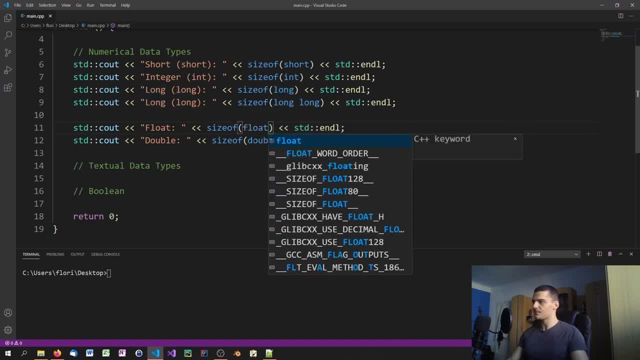 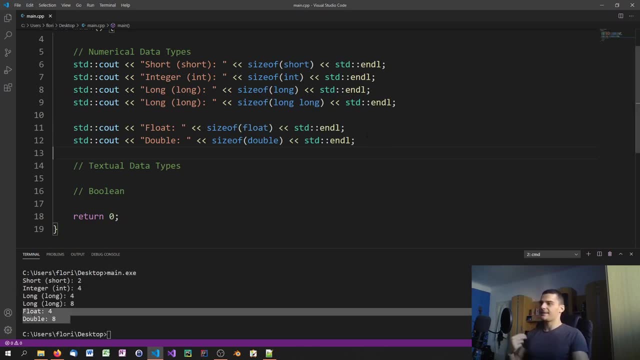 And the float has, I think, four bytes And we can see if that's true by just compiling and running. Yeah, as you can see, four and eight, And this means that the float stores up to seven digits of accuracy And the double, I think, was 15 digits of accuracy. 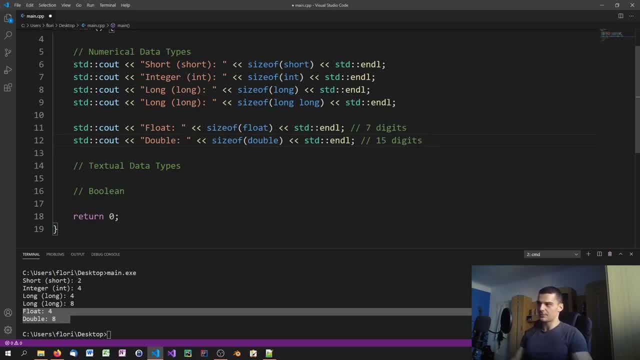 And, of course, if you need even more accuracy, what you do is you say long, double and then you have more accuracy. But yeah, this essentially means if you have a number like 16.7 or 16.75, you better store it in a float because it needs less memory. 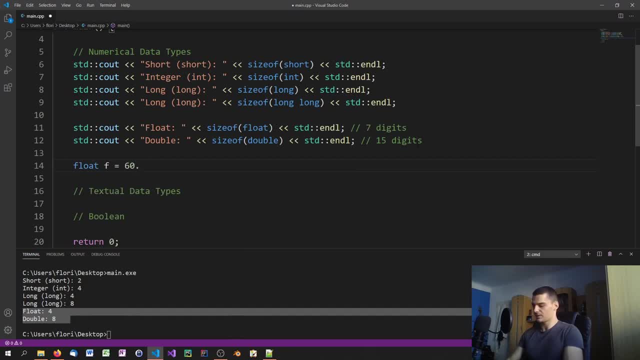 So we can say float f equals 60.78,, for example. And if you have a larger number, you say double d equals 90.8765.2.. And If you need even more than that, you just say: long double ld equals. 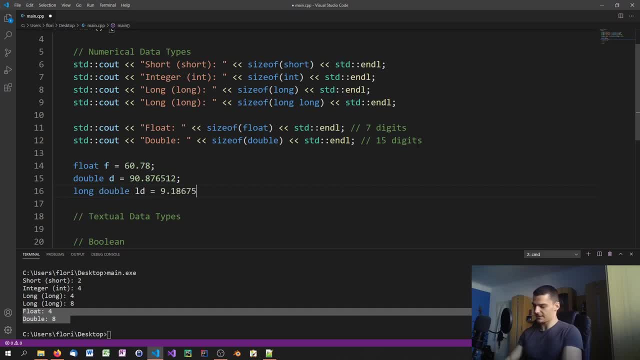 I don't know- 9.1867548976 and so on. So, depending on the accuracy you need, you choose the floating point value that you want to use. Now, before we get to the next data type category, I would like to show you something. 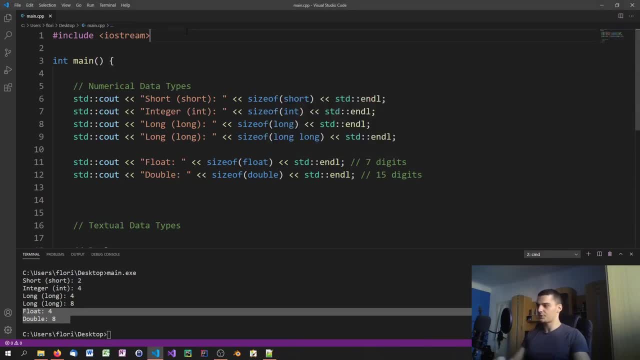 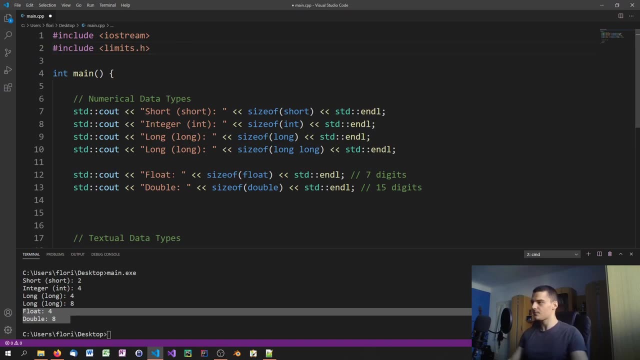 If you want to know the limits, the boundaries of a data type, what you do is you go ahead and include the library limit. So you say, include limits dot h, And when we have done that, we can use or we can access the maximum. 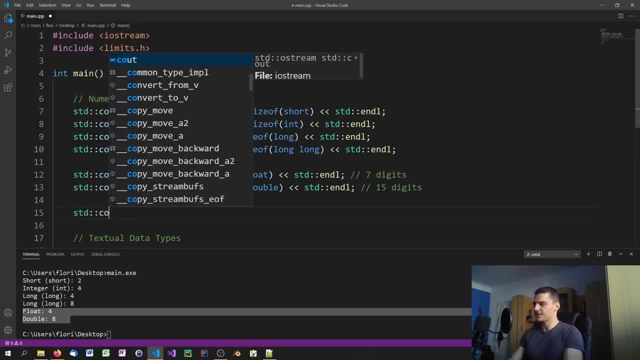 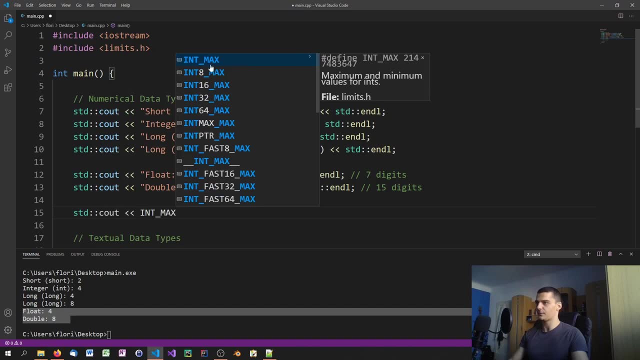 and the minimum values for each data type. So we can go ahead and say std cout And then we can say int underline max. This is the maximum value for an integer, at least for a signed integer, I think, If I'm not mistaken. let's see if that's true. 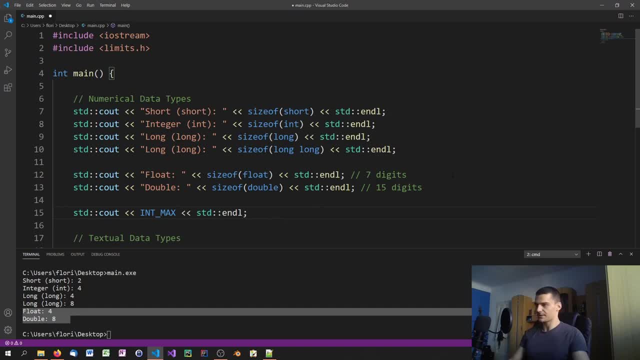 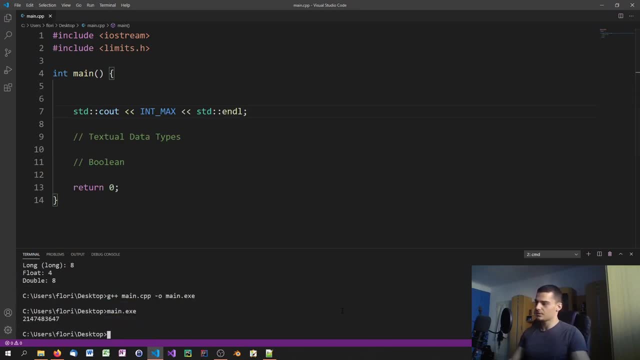 And we can go ahead and say std endline. Actually, let's get rid of all That's here. We don't need this anymore. And if we run this here, Yeah, it's a signed one. As you can see, it's half the actual maximum. 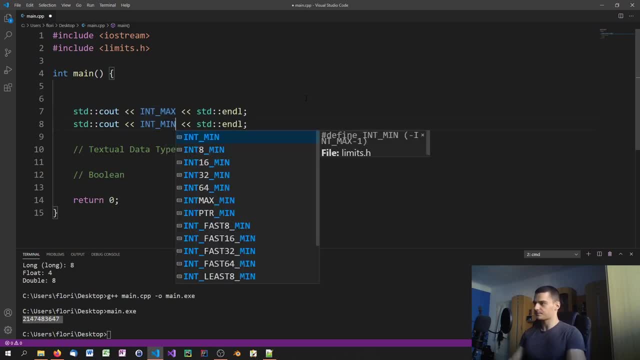 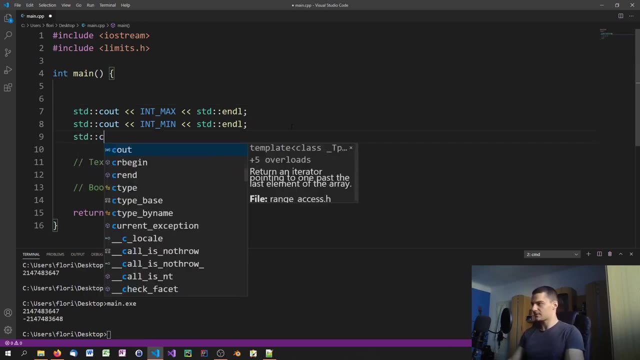 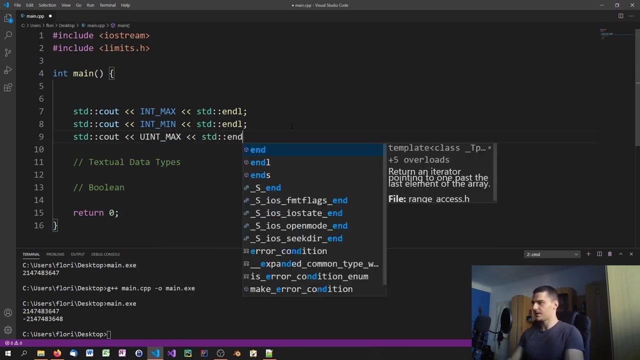 And we can do the same thing for the minimum here, Int min, And it works as well. Now I think we should also have something for the unsigned integer. So you int max std endline, Which stands for unsigned integer, And yeah, there you can see the maximum. 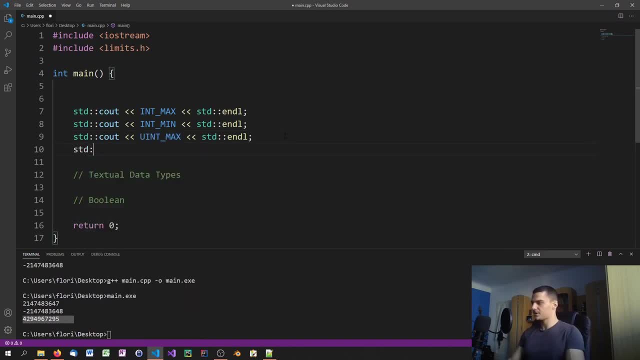 So if you want to access it real quick, you can do it like that, And I think this should be available for all numerical data types. So short, Actually, short is not available. Oh, actually, s h r t max is short. 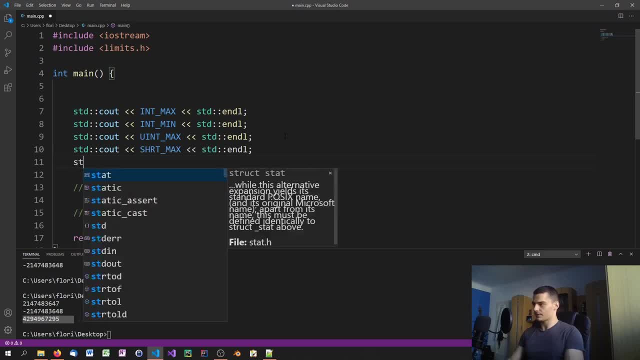 There you go, And it's probably also available for a long, So long, Long max And, as you saw, you also have long, long max. So we can see what that is End line, And let's see what we get as an output here. 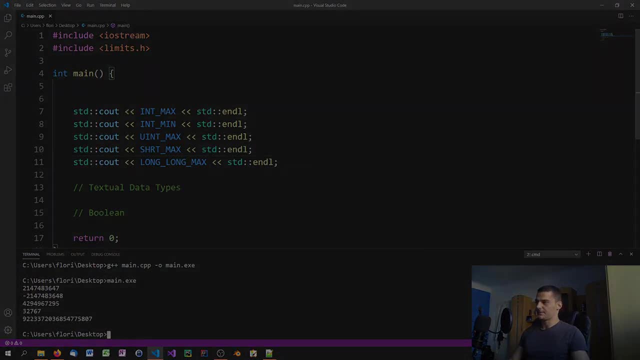 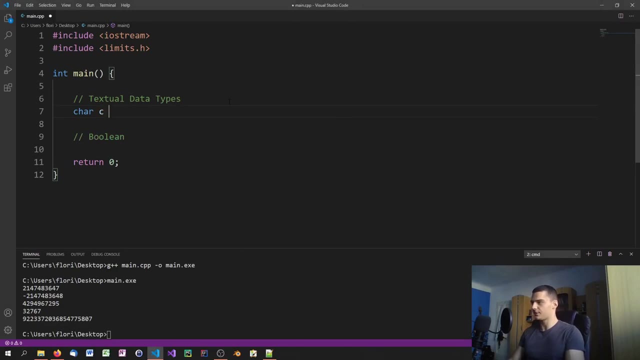 As you can see, this is the maximum value for long, long int. Great. So let's get into the textual data types, And the first one is the character, the char, The char c or character c. What we do here is we define a character by using a single quotation mark. 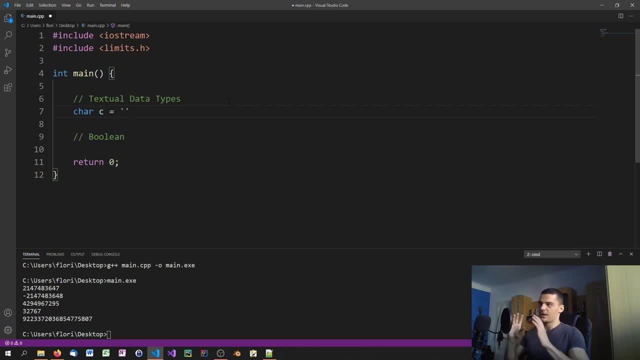 And this is just one Character. It's one character, I think character uses the UTF-8 encoding, which means that one byte is enough to represent all the UTF-8 characters. So a character we're going to see has one byte. 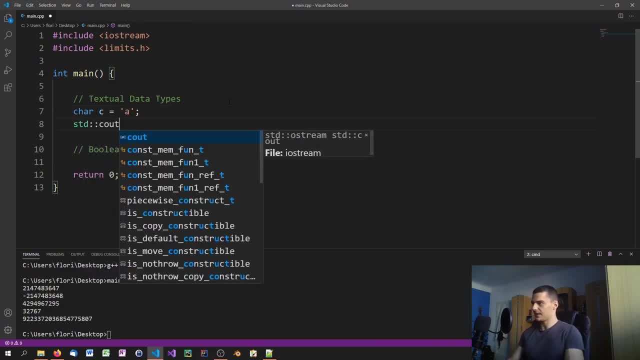 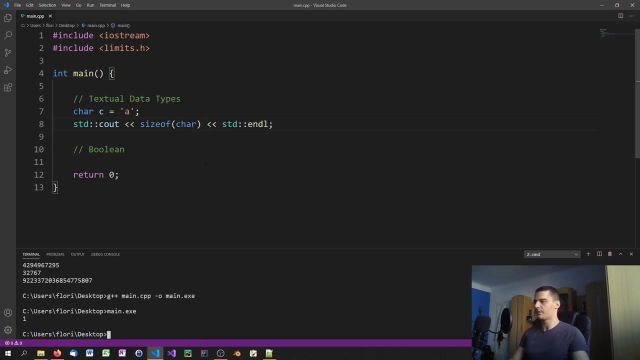 You can go ahead and print that std cout size of character And when we run this you will see it has one byte, which means four. Sorry, eight bit, Did I say four. But sorry, if I said four bit, I mean eight bit, of course. 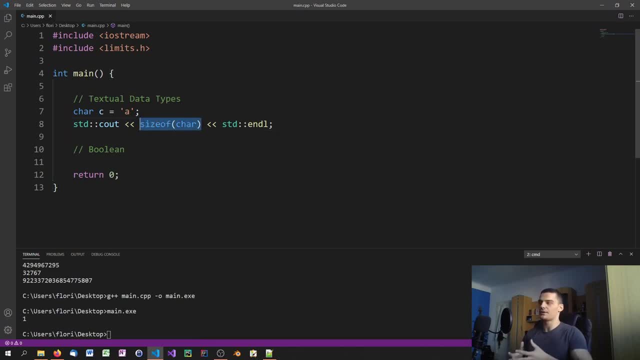 So this is sufficiently. this is sufficient to represent all the different UTF-8 characters, And we can go ahead and do it like that And you can see a, but I think we should also be able to assign a number like 19,, for example, and it. 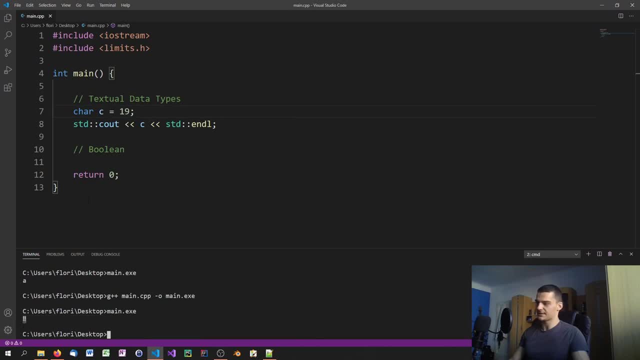 would typecast it into a character, As you can see. yes, 19 is this character? something like 80 should probably be a letter. Let's see if that's true. Yeah, As you can see, The uppercase P is the UTF-8 code 80, or maybe the ASCII code, but I think character is using. 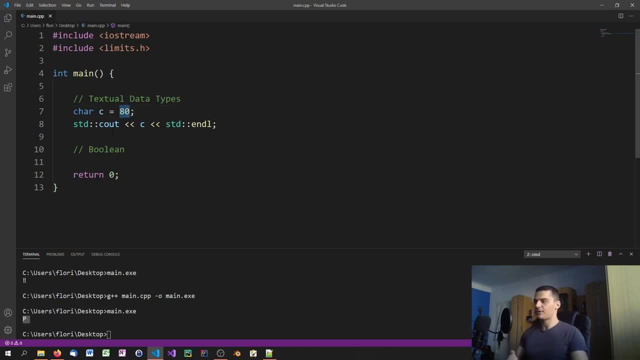 UTF-8 encoding here. So a character is just a number that represents a character. that represents a character And this character has a certain identification number. In this case, 80 is uppercase P, for example. That's a very simple data type, just has one byte and represents characters. 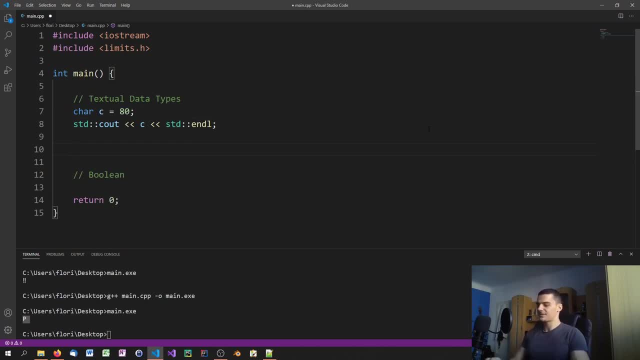 And now we have another textual data type, which is the string, And the string is actually just a collection of characters. Now, this is a little bit more advanced. You need to know about lists and arrays and so on, But a string is essentially just an array of characters. 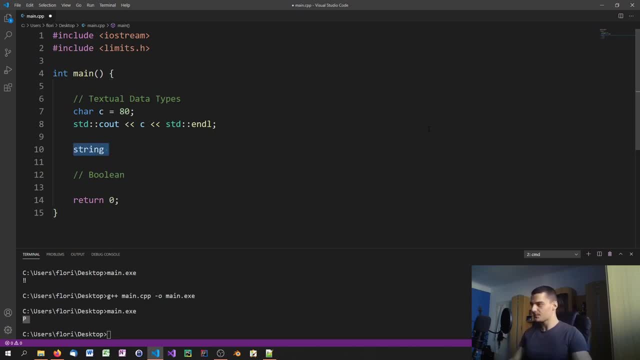 It's just a C array, a char array, so to say, But we're going to talk about that in a future video. For now, just use the std string And the string is just a text. The string is a text. 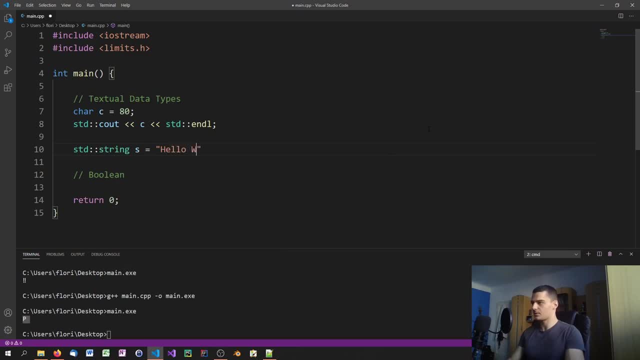 It has 24 bytes, I think. So hello world would be a string, And we can go ahead and print this String here And we can also print its size. I think it should be 24 bytes, if I'm not mistaken. 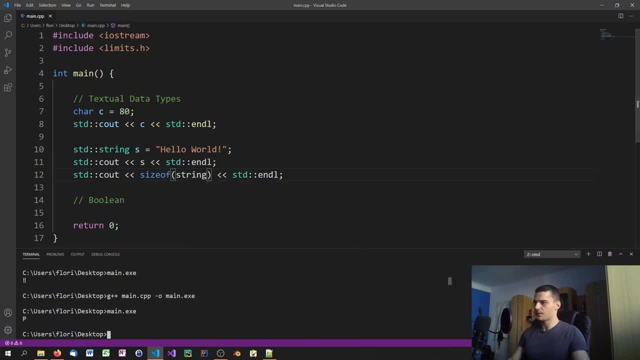 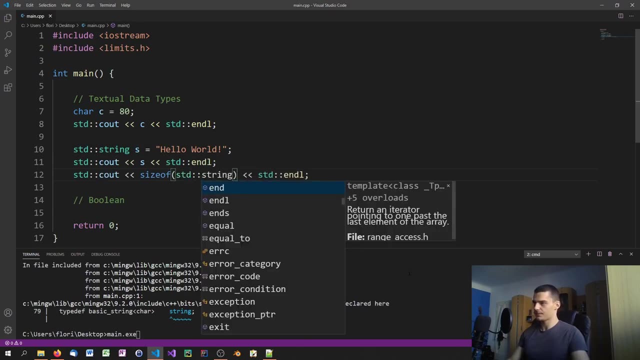 So size of string should be 24.. Oh, I got an error here. Oh, of course, Std string. Yeah, as you see, 24 bytes And hello world is a text. So whenever you work with text, you're using strings. 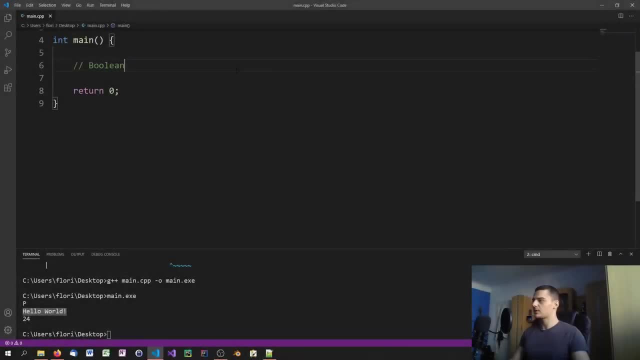 Individual characters. you use chars, Okay, So remember, we have different types of data types, So they're all being divided. We have the Boolean data type, the Boolean data type and the boolean data type. So the Boolean data type, we're going to call it boolean. 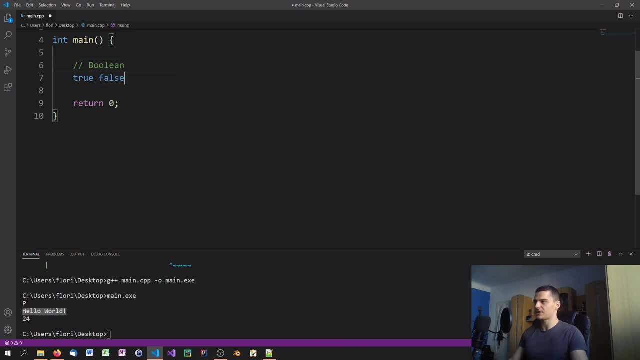 And we're going to call it boolean, And boolean is a very complex, very simple mean because it's a very complex parameter And we can define it in various ways. So let's create a Boolean that would be a Boolean hard drive. 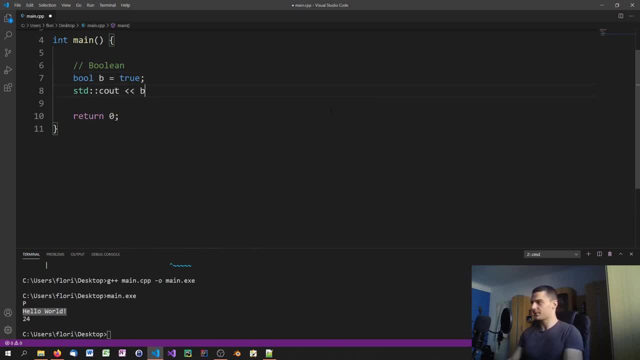 So let's create a Boolean driver And this is a Boolean table. So at the end of the bio it's what and line, And you'll see that we get one. this is important because, even though we have the keyword true, a Boolean is just one or zero, So we can treat it as a number like, not necessarily. 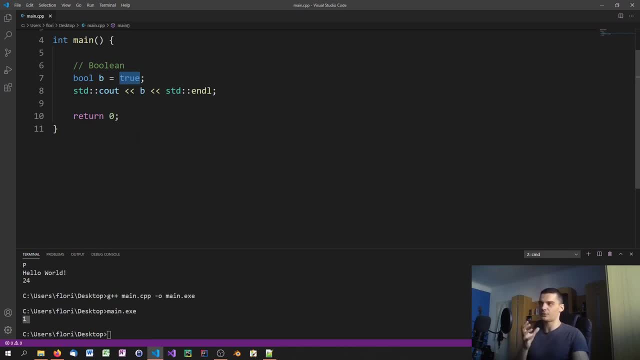 a number that you can do calculations with, but you can check for zero or one. you can also define it by saying: bool b equals zero. this would be false And it will also print zero, of course. but it's not all of a sudden an integer, right? It's not just an integer or a short that you can. 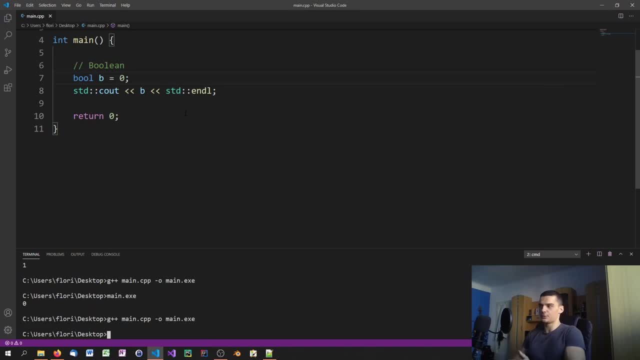 do calculations with. it's zero or one. it's a Boolean value. it's true or false. It's also represented as zero, zero and one, but it's still true or false. And this is something that we're going to need when we get to conditions, when we get to comparisons, when we want to know. 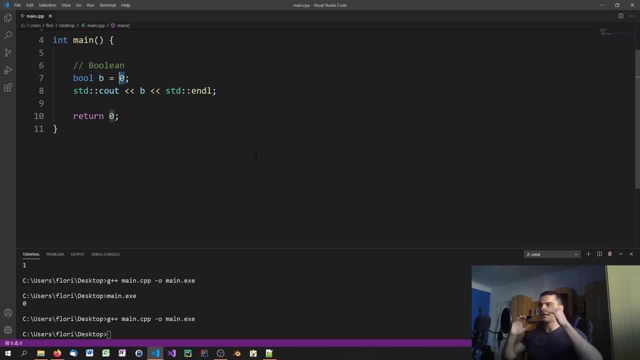 if something is true. you know, in programming you have certain conditions where you can say: if something is true, do that, otherwise do that. And the value that this comparison- if something is true or this statement- gets you is a Boolean value. So when you try to say 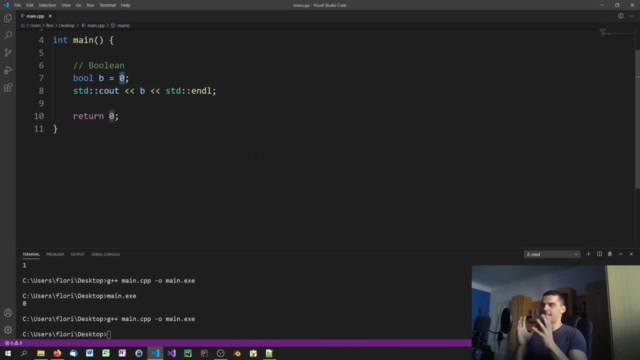 if the input of the user is valid- this is a Boolean value: the input is valid, true, the input is invalid, false- or if this number is less than this, and this is also a comparison that gives you a Boolean which is either true or false. So this is a very important data type. 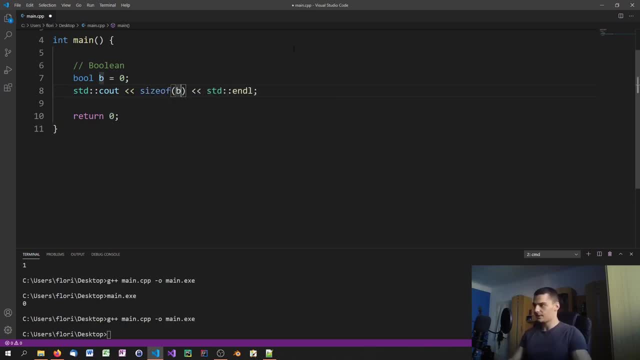 we can also look at the size of it. as I said, it's one byte, Not clear screen. come on, compile main access, as you can see one byte. By the way, one thing that I didn't mention here is that you cannot only get the size of the data type itself, you can also. 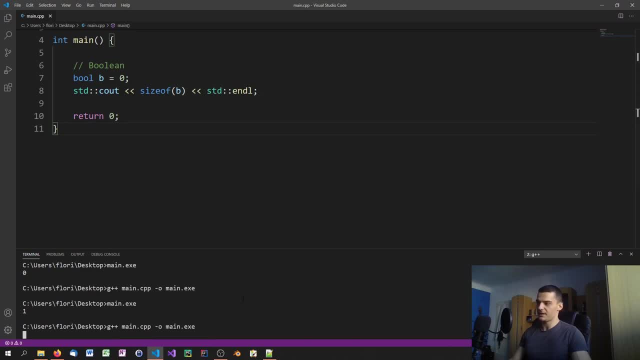 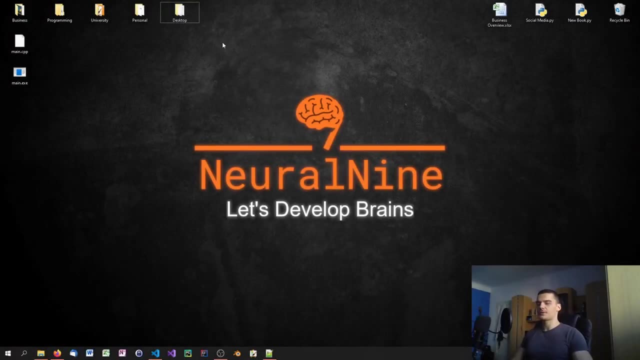 say, get the size of B, which will be the same in this case, but sometimes it differs, So you can also get the size of a particular variable. Alright, so that's it for today's video. I hope you enjoyed it. I hope you learned something. If so, let me know by hitting the like button and. 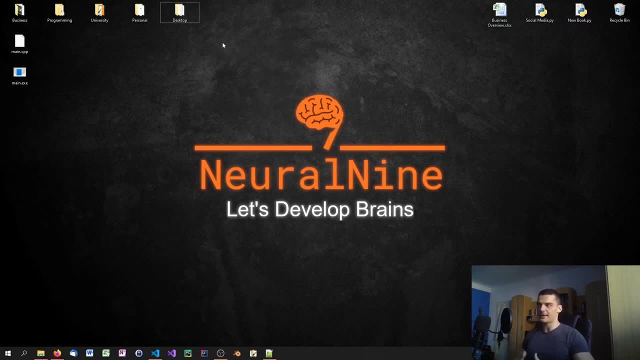 leaving a comment in the comment section down below. I tried to cover everything here in as much detail as possible. I hope you enjoyed it. I hope you learned something. If so, let me know by hitting the like button and leaving a comment in the comment section down below. I tried to cover everything here in.